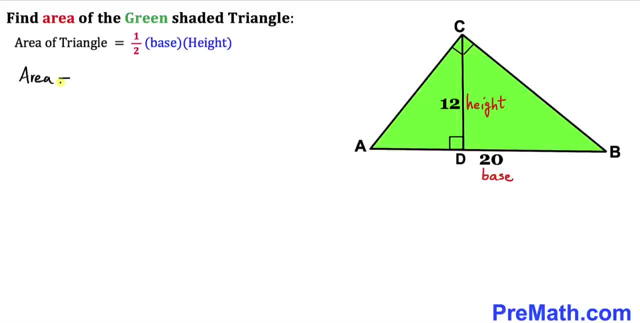 area of this triangle ABC is going to be a half time, base is 20 times height is 12 and if we simplify everything, we are going to get 120 square units. however, this is not a correct answer, so this is wrong, but why? now I'm going to show you why this. 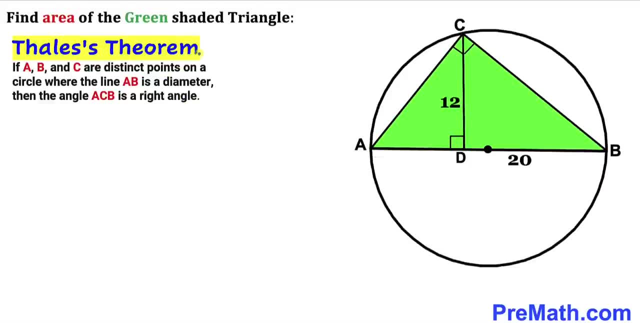 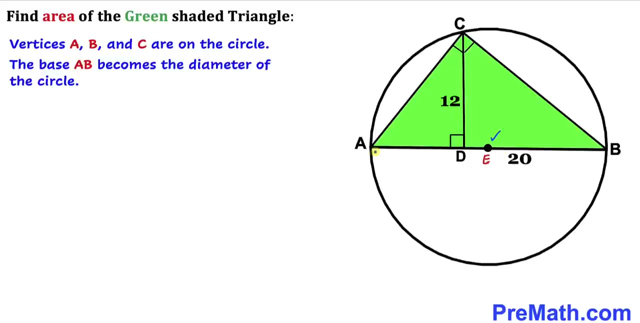 is not possible. and now let's recall the Thales theorem. according to this theorem, these points- AB and CR on the circle and, moreover, this base, AB is the diameter of this circle and, moreover, E is the center of this circle, such that this a, E and e, B are the radii of this given circle. and the radius. this one is going to be D and the radius of this circle is going to be Ds, because A and C, for whatever reason, we are not the limits. so we just have to say: if AB is the center on встречable area, columell on the circle. These points. let us compare the scope work sister asking: can this problem? and in this case let us give differences. the rumble there, So twenty-five points each coconut if we divide theAll right. so c plus bxc, equal morning. or the method ofaces of Currie batch is two. now let's think one more time, and this is one of the things that the 고 er well, and liza will. Chandler will conclude with thisget a really good idea here. 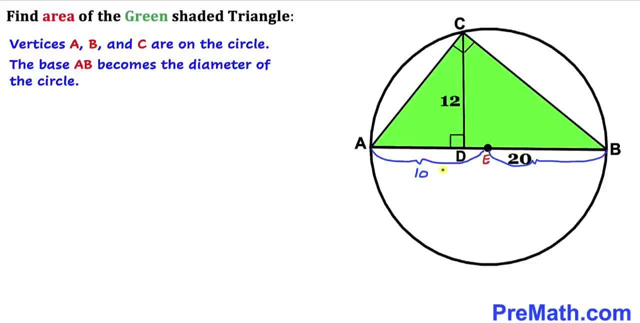 to be half of this diameter, 20, so that's going to be a 10 units, and this radius is going to be 10 units as well and, moreover, this EF is going to be the radius of this same circle as well and its length is going to be 10 units. and now we can see, in reality, this radius EF is bigger in length. 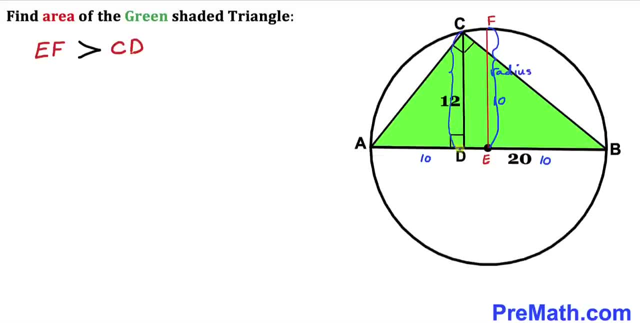 than this height CD. and here we can see our. this EF length is 10 and this CD length is 12. therefore we can see that 10 is greater than 12 is a false statement and that's impossible. so therefore we conclude that this height CD cannot. 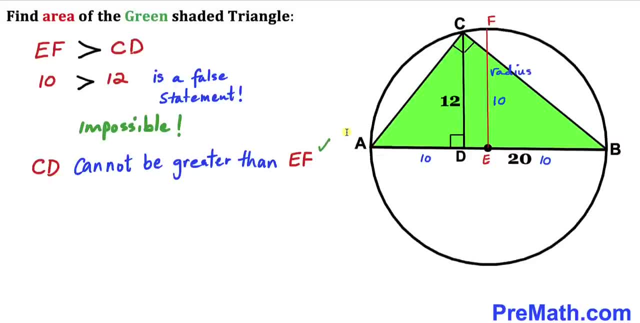 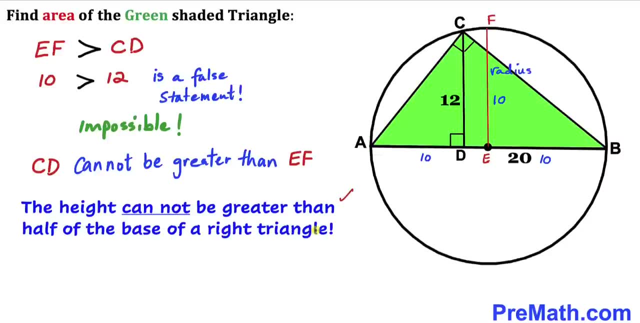 be greater than this height CD. and therefore we can see that this EF length is greater than this radius EF. and here's our bottom line: the height cannot be greater than the half of the base of a right triangle. and here's our conclusion: no such triangle exists because 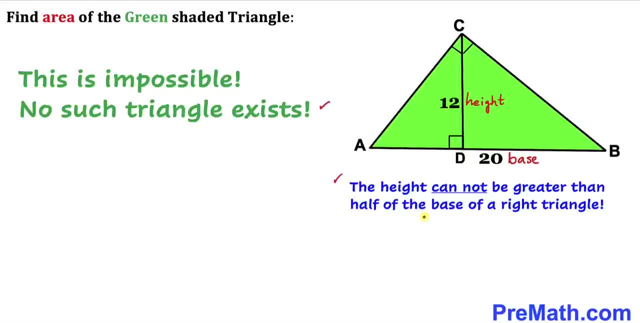 the height cannot be greater than the half of the base of the right triangle. thanks for watching and please don't forget to subscribe to my channel for more exciting videos. bye you. 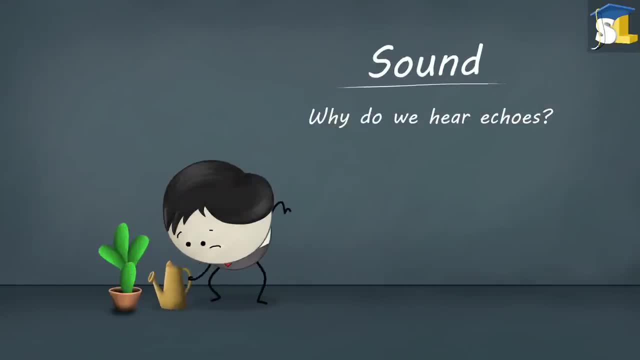 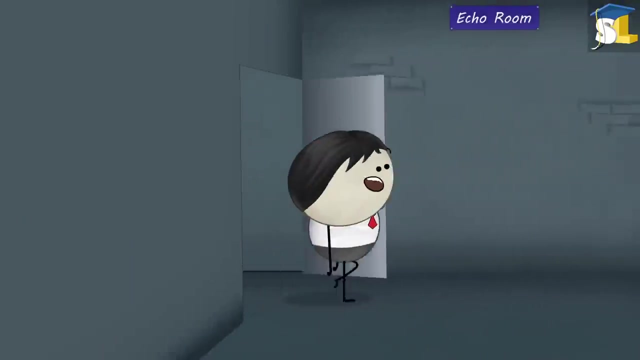 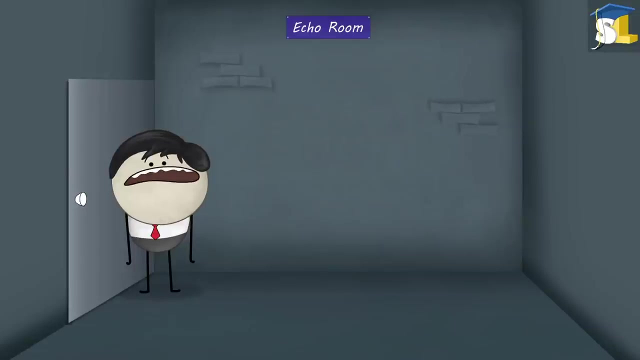 Sound? Why do we hear echoes? Hey, hold on, Don't go into that room. You don't want to listen to me? Okay, Then go ahead. See, I warned you. Will you listen to me now? Don't worry. 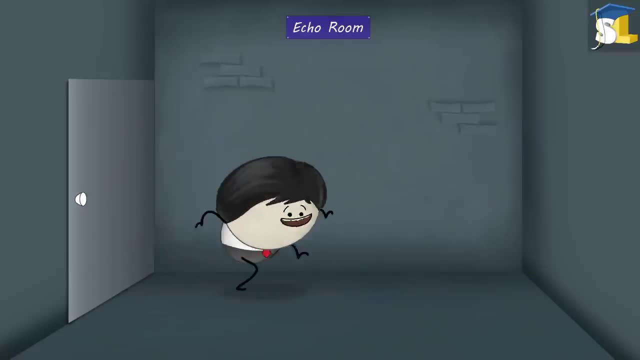 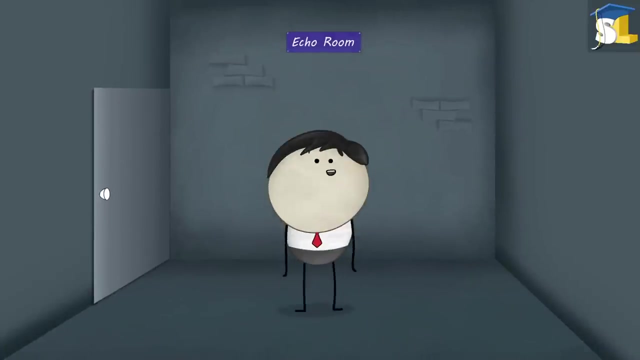 The sound you heard was just an echo of your voice. Let me explain what an echo is. When we speak or laugh in a big empty hall, we hear our own sound repeatedly. This is because our sound waves get reflected from the walls of the hall back to us. 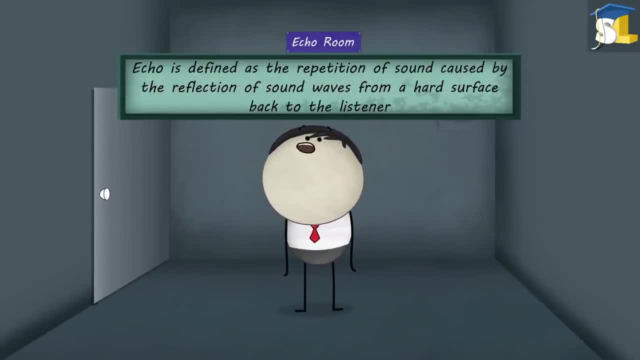 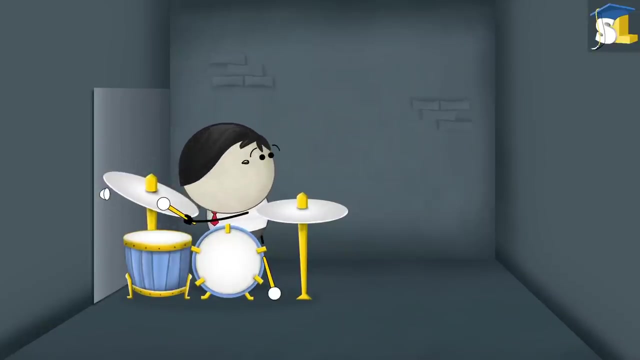 The reflected sound that we hear is called an echo. Hence, an echo is defined as the repetition of sound caused by the reflection of sound waves from a hard surface back to the listener. This is because the visible echo is not a sound wave. Hey, what are you doing? 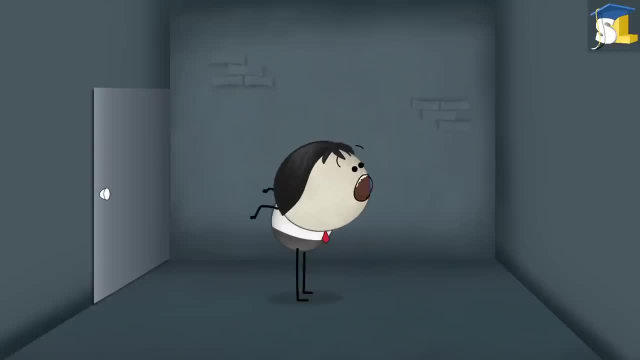 Are you trying to hear an echo? It is not that easy. There are two ideal conditions for an echo to be heard. When we speak or laugh, we hear our original sound. at that moment. The sensation of this original sound remains in our brain till 0.1 seconds. 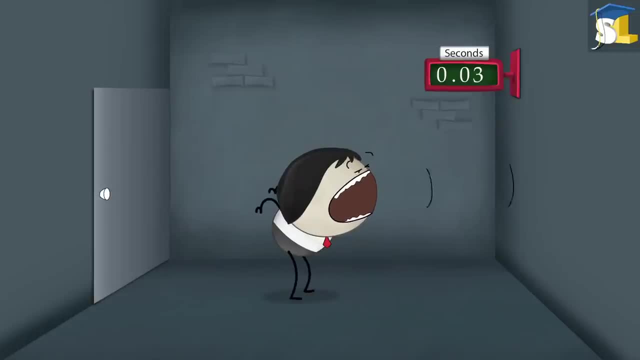 When we utter sounds, some of our sound waves get reflected, while some get absorbed. If the reflected sound waves reach our ears before the completion of 0.1 seconds, Then our brain does not perceive the original and reflected sounds as separate sounds. They are interpreted as one sound. 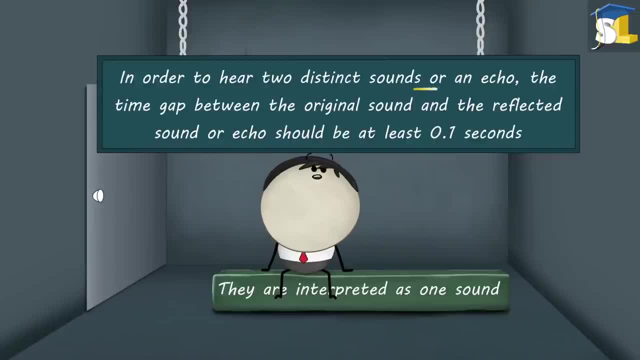 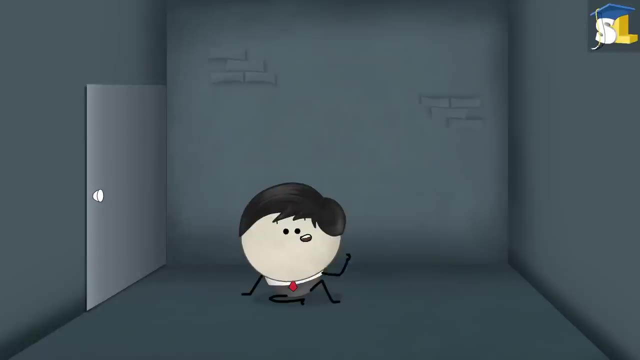 Therefore, in order to hear two distinct sounds or an echo, The time gap between the original sound and the reflected sound or echo Should be at least 0.1 seconds. This is the first condition for an echo to be heard. Do you know when the time gap will be more than 0.1 seconds?